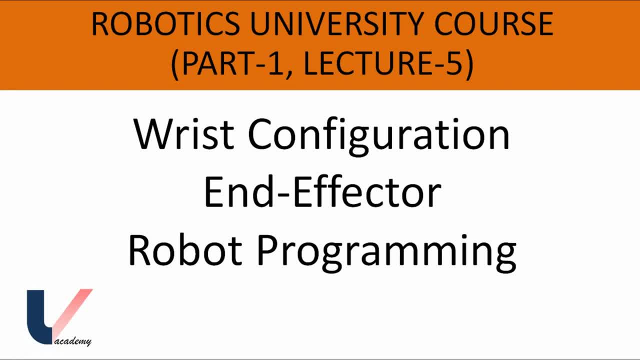 Hi, welcome back to the Robotics University course. Till now, we have studied about two main parts of a manipulator, that is, links and joints. In this lecture, we will be studying about two other main parts of a manipulator, that is, wrist and end effectors. Apart from this, we will study another. 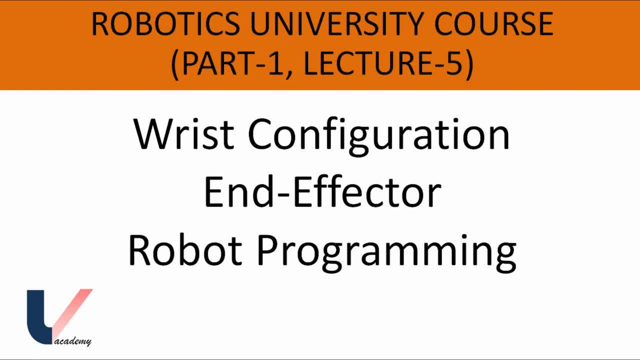 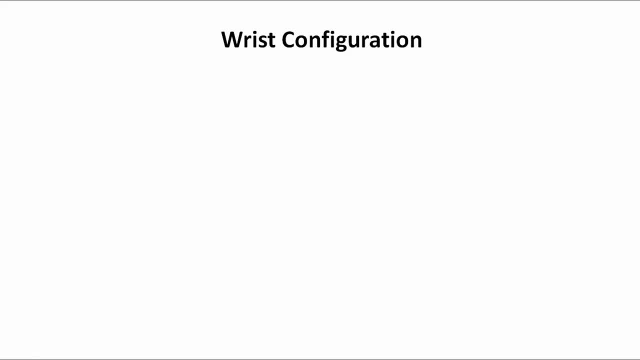 important topic that is, robot programming. So let's start with wrist. Arm is the first section of the manipulator and wrist is the second section of the manipulator. Wrist is attached at the end of the arm. Wrist is used to orient the end effector in 3d space For orientation. 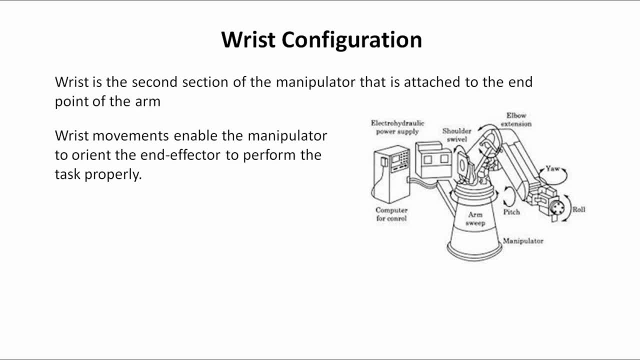 in any way in 3d space. the wrist requires three degrees of freedom. that gives three rotations about three principal axes: The x-axis, y-axis and z-axis. But depending upon the application, as how we want to orient the end effector, the degree of freedom. 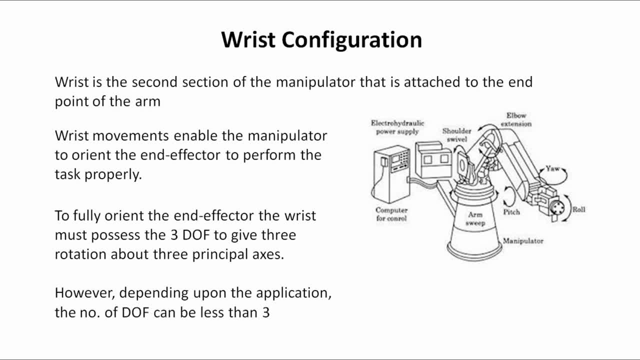 can be less than three. Okay, depending upon the application. suppose there is an application where only two degrees of freedom are required, So the mechanical design of the wrist will be according to the two degrees of freedom. Okay, moving further, the three rotations of the wrist are known as roll. 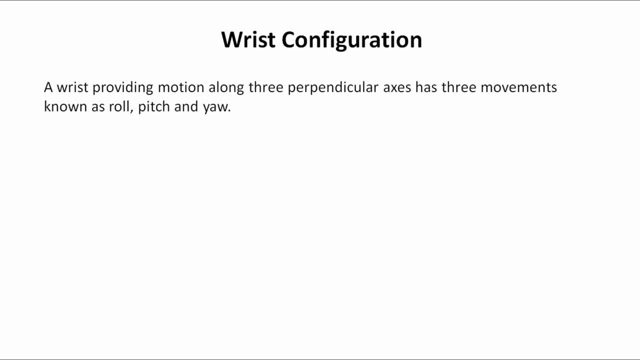 pitch and yaw Roll is the most common rotation of the wrist. The most common rotation of the wrist is the motion in a plane perpendicular to arm end, As shown in the diagram. you can see that roll is the rotation about the horizontal axis in this way. Similarly, pitch is the motion in the vertical. 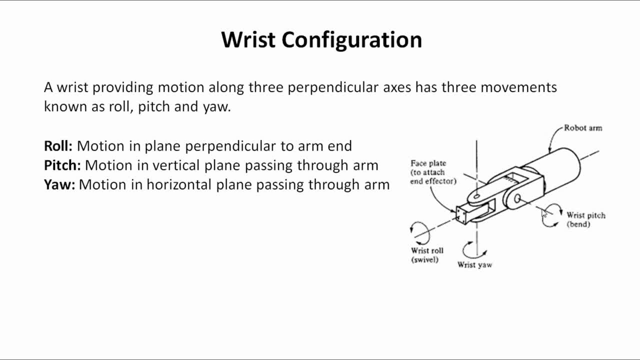 plane passing through the arm That is pitch is the rotation about the another horizontal axis as shown in the diagram. The third motion is yaw. Yaw is the motion in the horizontal plane passing through the arm That is. yaw is the motion, the rotation about this vertical axis. 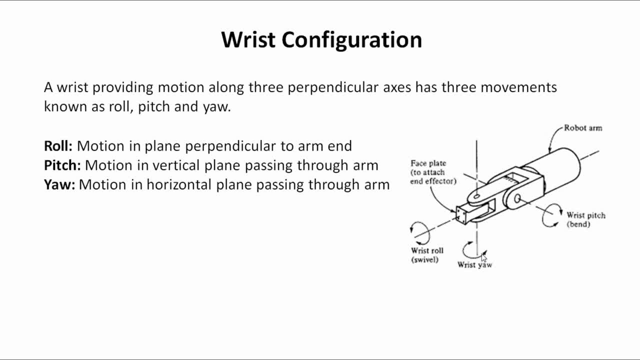 A wrist with high dexterity is the one where three axes intersect at a point. If the three axes intersect, such a wrist will have high dexterity. Okay, in robotics we have seen that as the dexterity is increased, the complication in mechanical design also increases. So we have seen that the 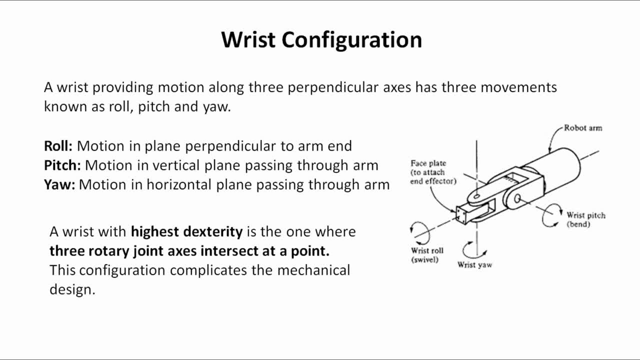 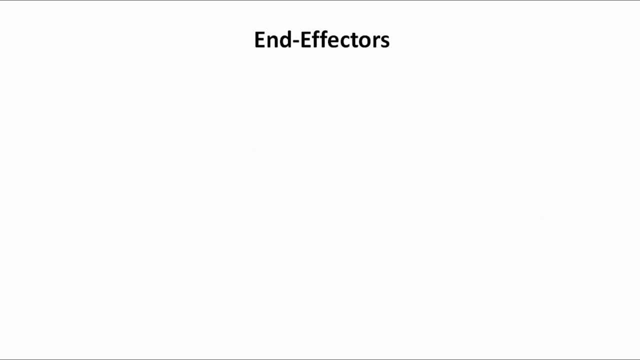 wrist with high dexterity increases, So in wrist also. if three axes intersect, the mechanical design will become complicated, Moving further. the last part in the study of manipulative is end effector. These are attached at the end of the wrist and are used to perform a specific task. Okay, one important. 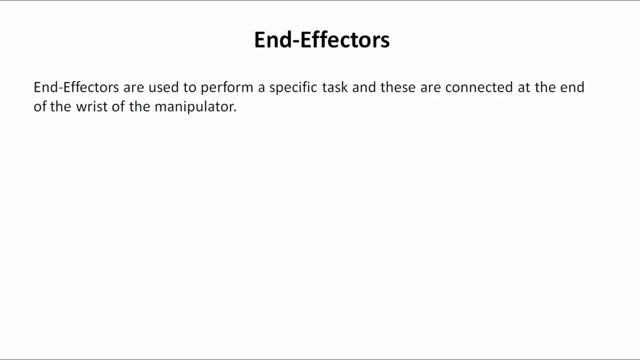 point to be noted over here is that the end effector are external to the arm. These do not add to any position. These are external to the arm. These do not add to any position. These are external to the arm. These are external to the arm. These do not add to any position. These are external to the arm. 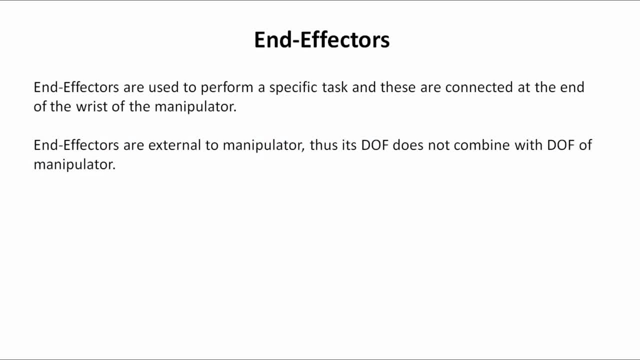 These do not add to any position. These are external to the arm. These are external to the arm. So the Почему these are external to the arm secretion is partially dependent on the degree of freedom of the end effector, which is in winds direction of the arm and in Christians vision. 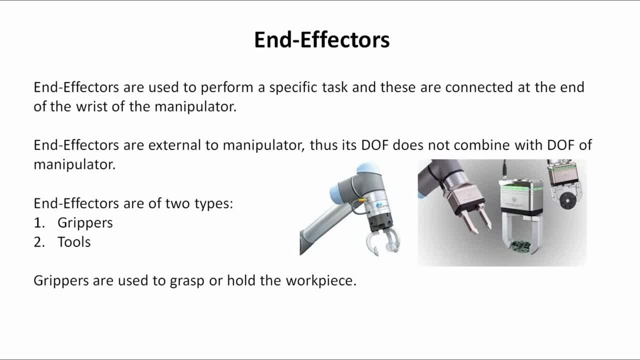 are the jeers of freedom of the manu, The end effector adjacent to the arm, at the arm center, are way further a distance adjust to where the end36, so to say, greater than the worse, waiting between the direction of the arm in which the arm itself is placed and theία to which this English wasyers all. 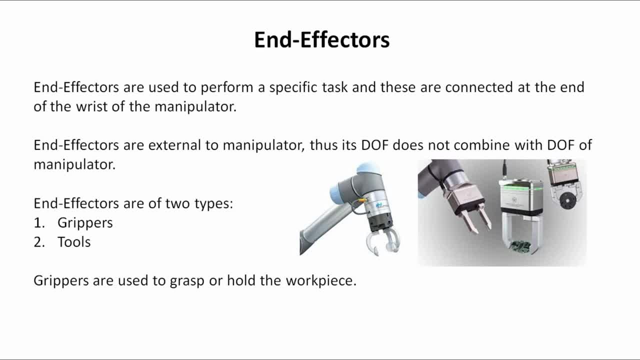 three axes are peculiar to any mechanical people. so two such degrees of freedom are moreowie have to be. freedom of the end effector are not combined with the degree of freedom of the manipulator. These end effectors are of two types. First one is grippers. Grippers are used to grasp or hold. 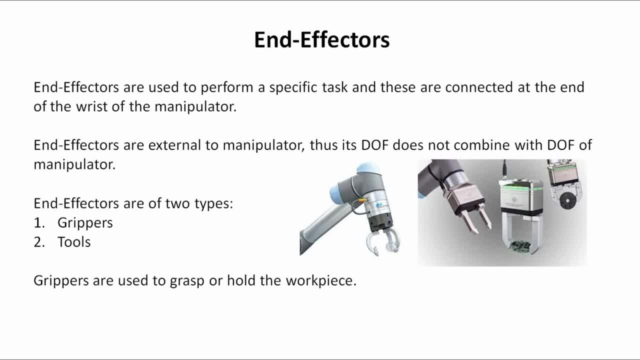 the workpiece or tools, And the second type of the end effector is the tool itself that can be used to perform various tasks like welding, grilling, grinding, etc. So we have completed the study of basic structure of the manipulator. Now we will study about robot programming. 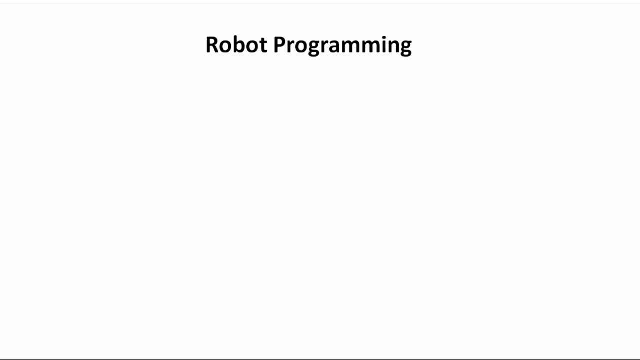 Robots are required to do some work cycle. But robots have no intelligence of their own. They need to be taught as how, when, where and in what sequence to do a particular task. The teaching of the work cycle to a robot is known as robot programming. 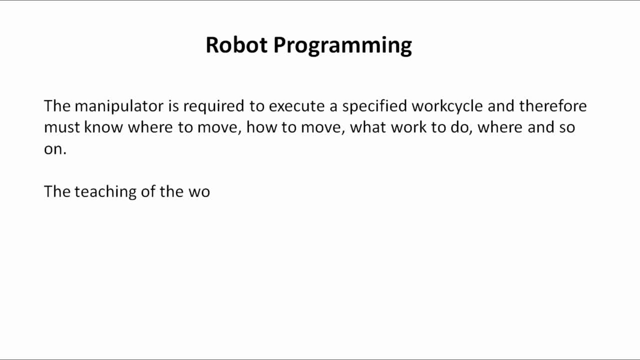 Now, robots can be programmed in two different ways. Number one: teach by showing or lead through programming. Number two: textual commands with a suitable interface. So the first one: teach by showing or lead through programming. In this method, the manipulator is made to move through the desired motion path of the